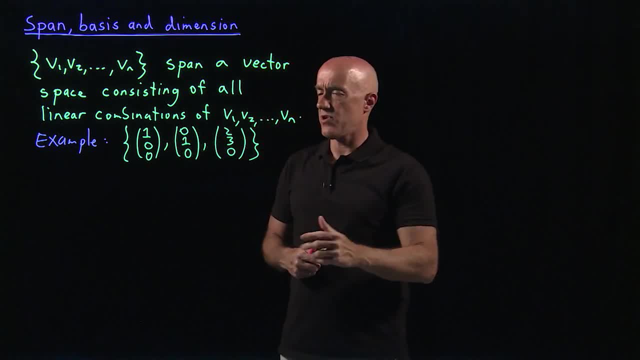 So these are three vectors. They're 3 by 1 column matrices. These three vectors span a vector space, So all linear combinations of these three vectors will span the vector space that has 0.. The vector space actually is 0.. 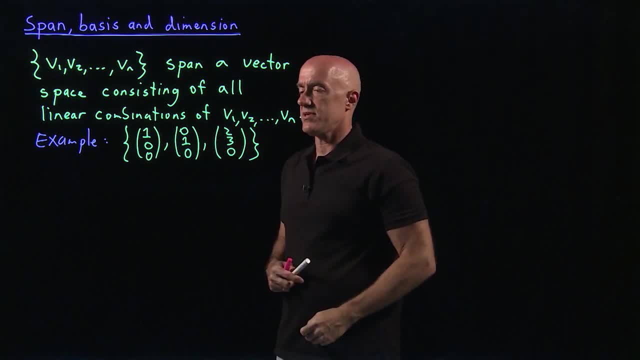 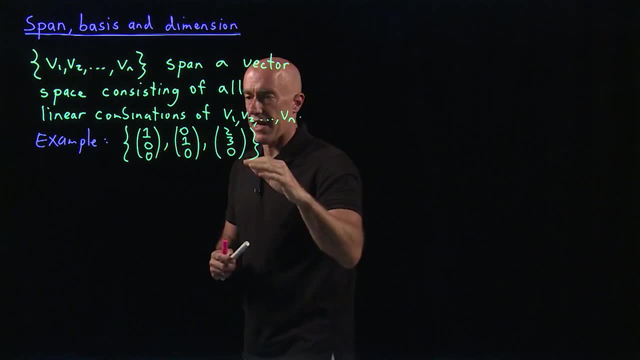 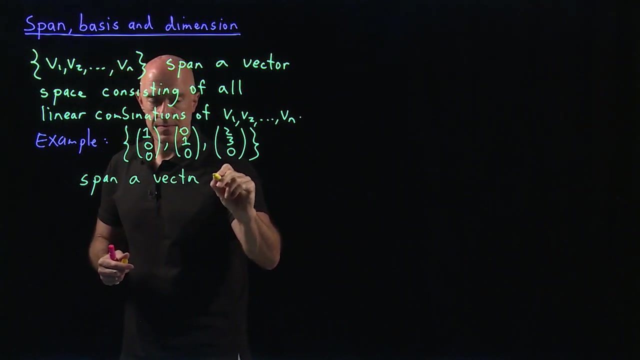 So the vector space is actually consisting of 3 by 1 matrices that have 0 in the third row right. So this is the vector space. These span a vector space of 3 by 1 matrices with 0.. OK. 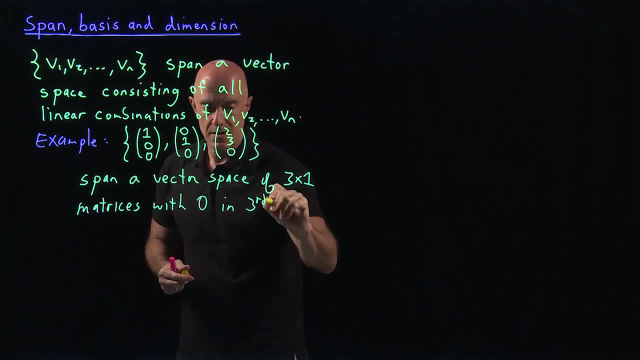 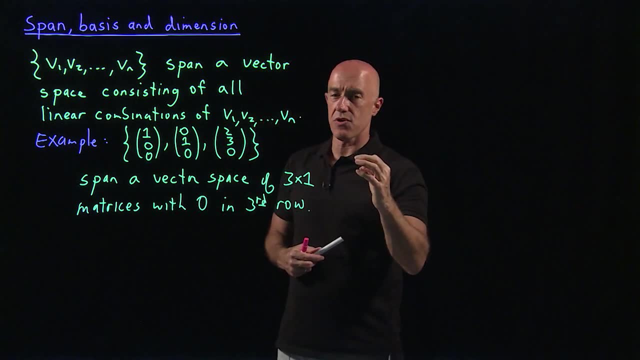 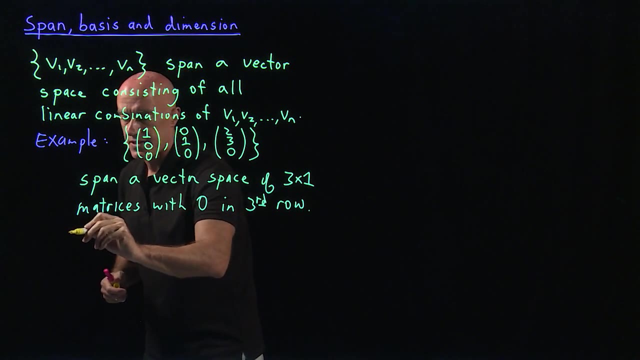 OK, OK, OK. So we get 0 in the third row right And we say that that's also a vector subspace. So that's another definition. So this vector space, this is a vector subspace of all 3 by 1 matrices. 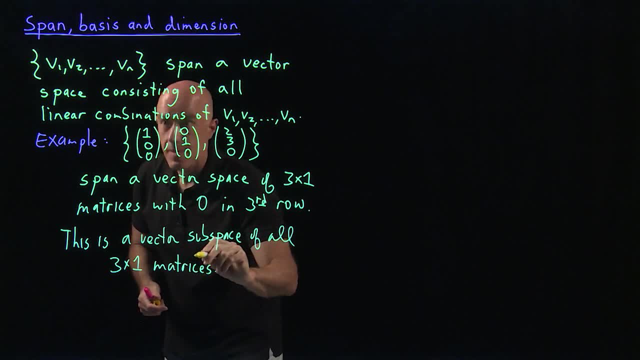 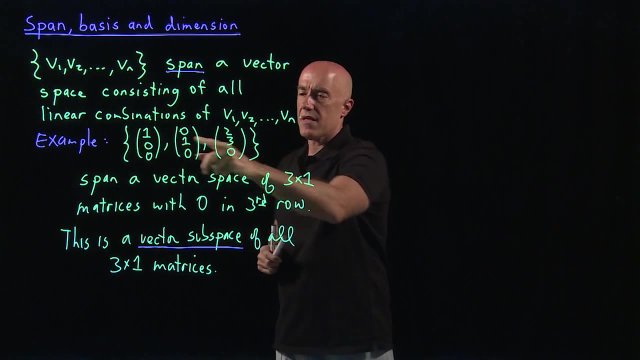 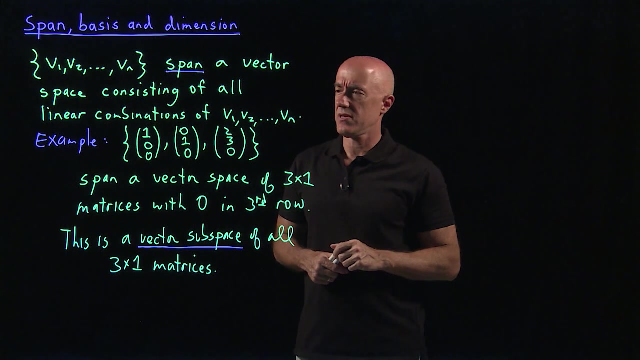 So here I define span and I define the meaning of vector subspace. If you look at these three vectors you would say, okay, we're spanning a vector subspace that has zero in the third row. but do we actually need all these three vectors? 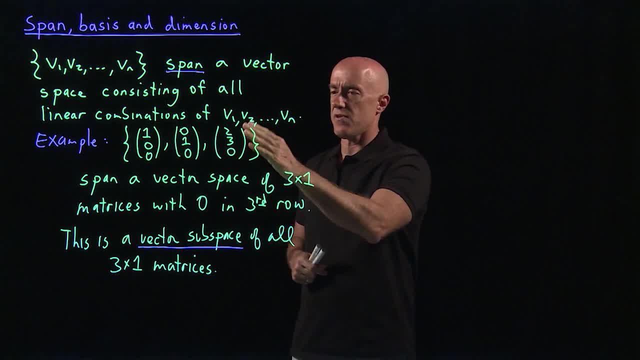 No, because in the last video I showed you, the third vector is a linear combination of the first two, so that these three vectors are not linearly independent. they're linearly dependent. So in fact, we only need two of these vectors, and that's the definition of a basis. 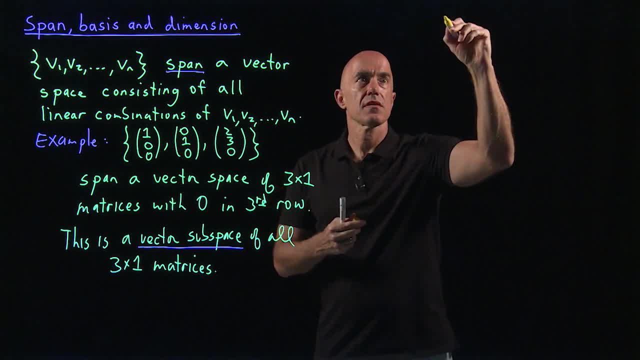 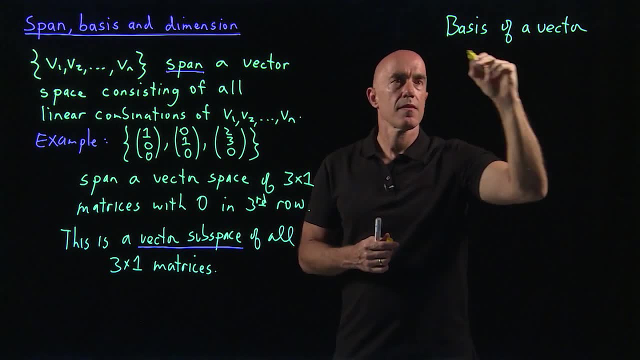 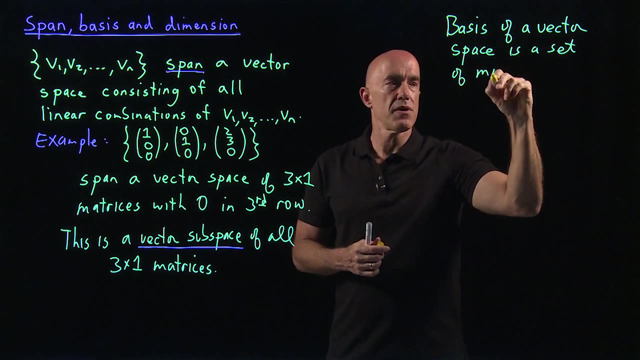 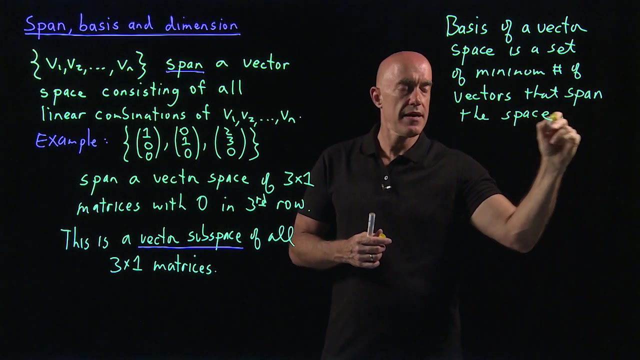 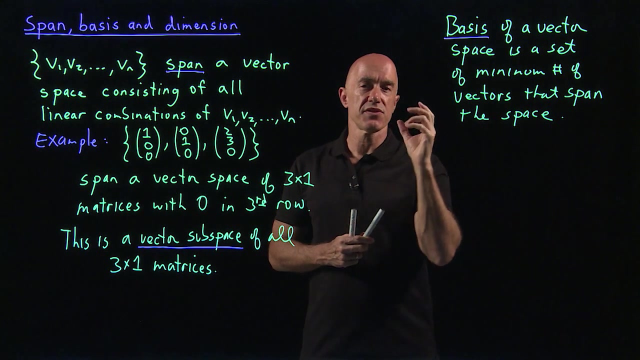 So a basis of a vector space is a set of minimum number of vectors that span the space. Okay, So that's the definition of a basis for a vector space. So it's the smallest, so it's the number, it's the vectors that can form a smallest. 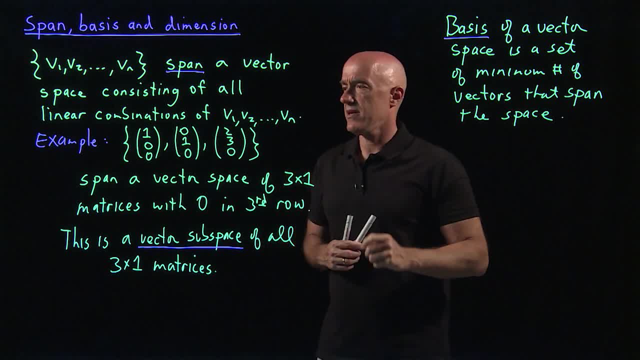 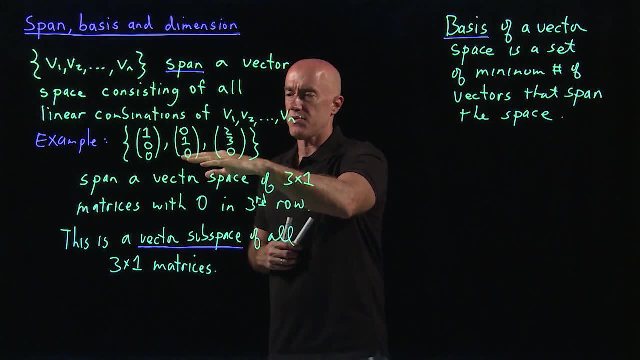 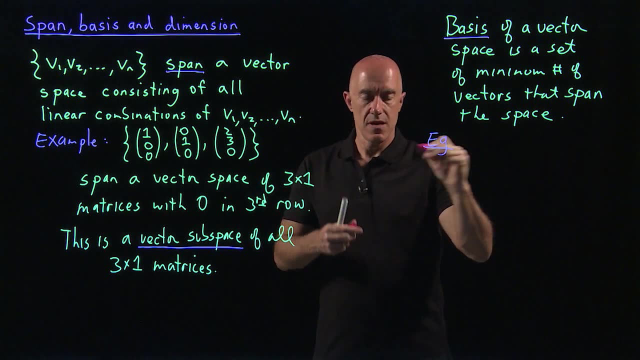 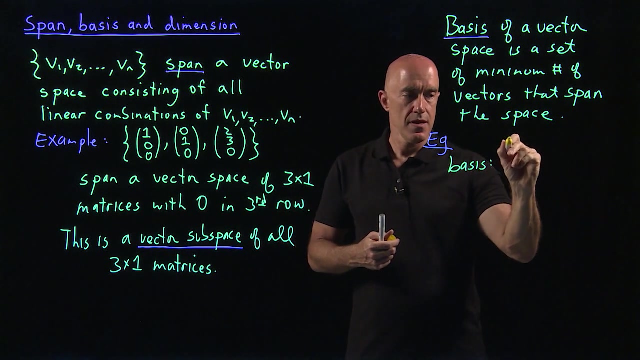 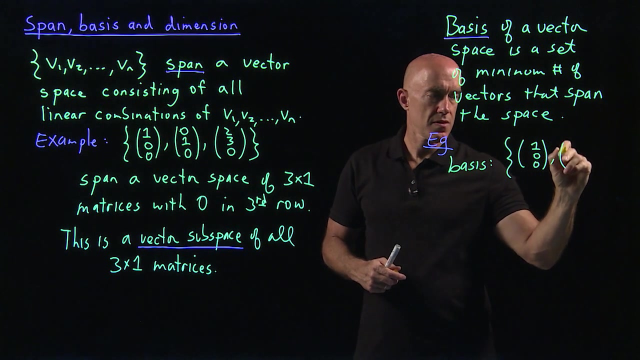 set that can span the vector space. So here the vector, the basis for the vector space consisting of three by one matrices, with zero in the third row. so as the example here, The basis could be the following: It could be just the first two vectors, right? 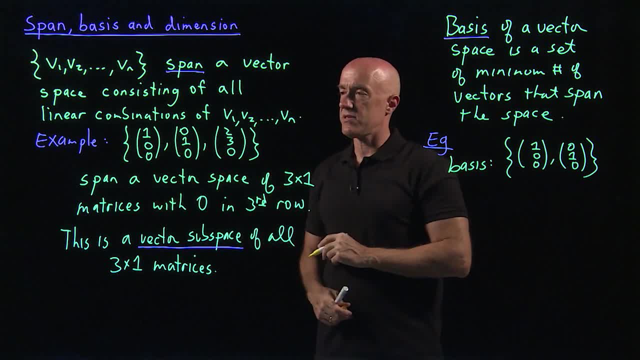 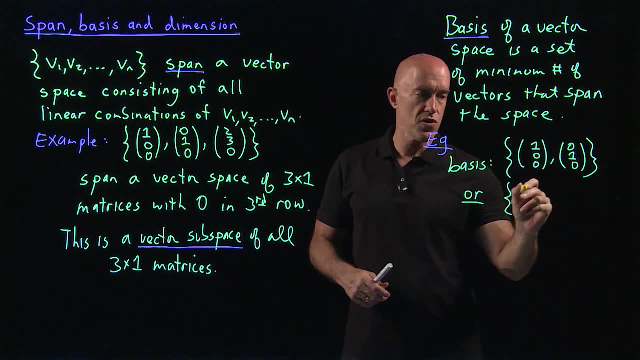 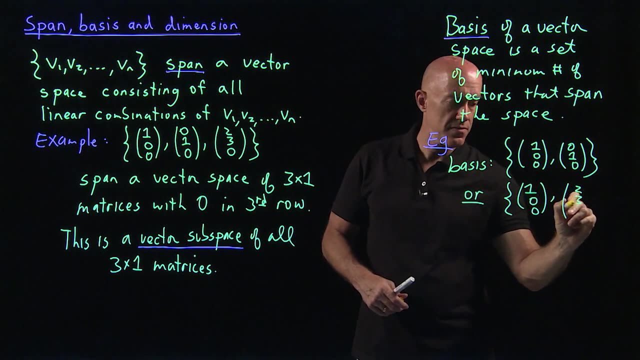 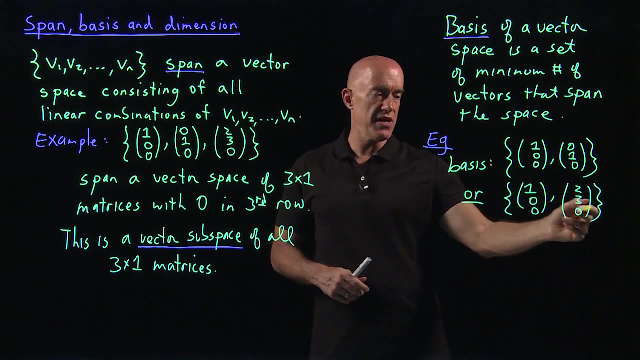 That forms a basis for this vector subspace or this vector space. but we could have any of these two vectors, So it could be one zero zero, two, three zero. That can also generate all three by one vectors with a zero in the third row. 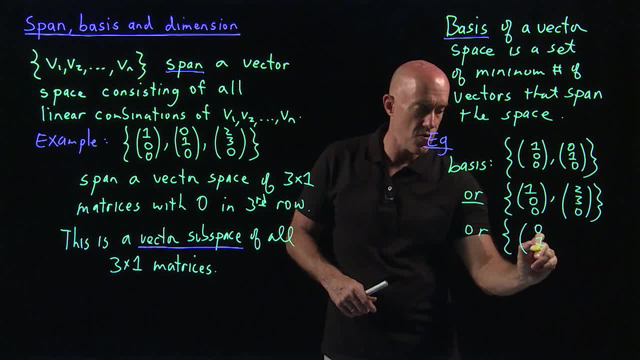 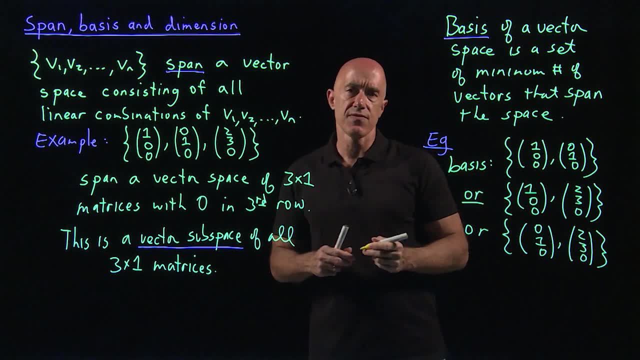 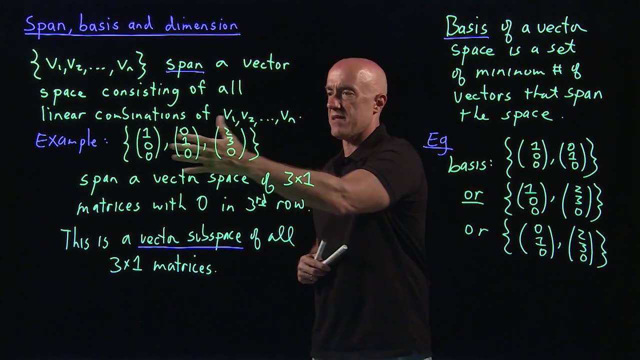 Or we can even have the other combination: zero, one zero and two, three zero. So these three sets of two vectors, All four, form a legitimate basis for the vector space spanned by these three vectors. We'll see that we're going to actually 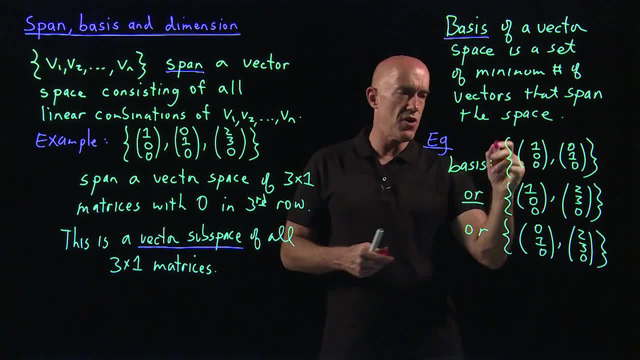 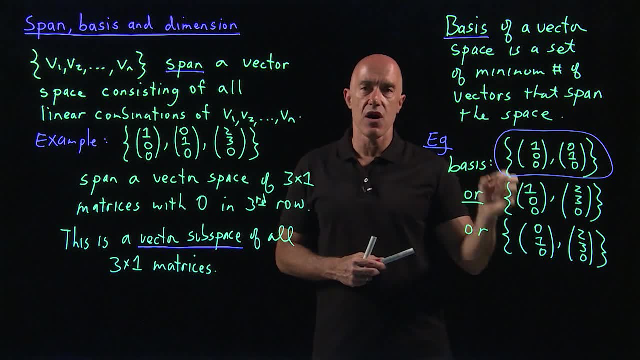 prefer one of these sets, We're going to prefer the first one if we have a choice between these three, because these vectors are orthonormal and we're going to like orthonormal, So orthonormal means that. so let me put the word here. 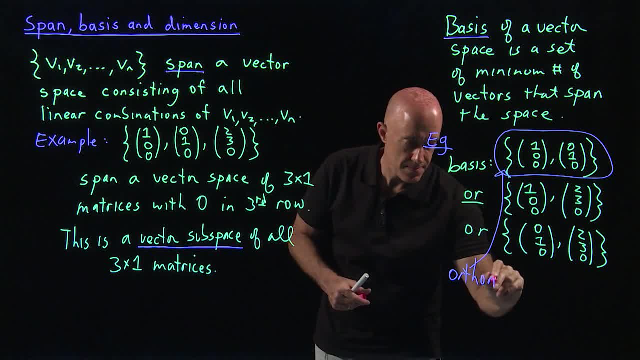 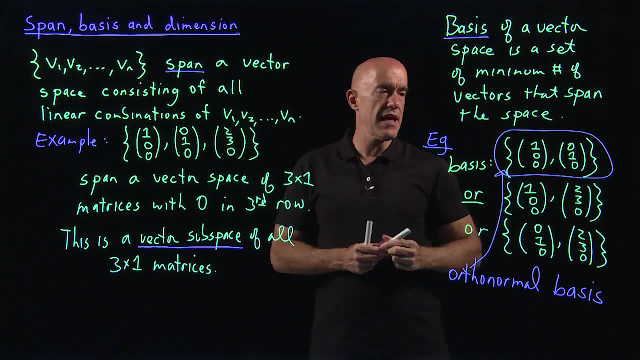 So these are orthonormal. So we say it's an orthonormal basis. It means that these two vectors are orthogonal. So 1, 0, 0 transpose 0, 1, 0 equals 0, right. 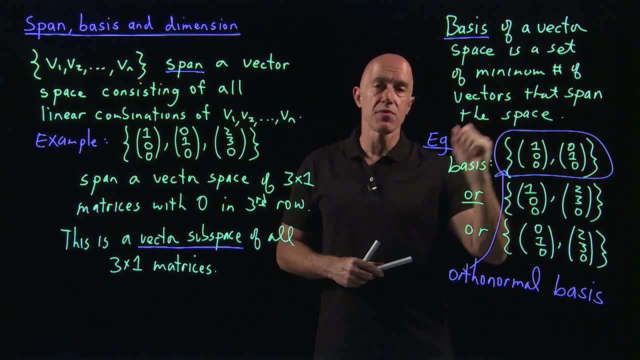 That's the dot product And they're normalized, So 1.. So we say that these two vectors are orthonormal. This is an orthonormal basis. There are other orthonormal bases, but this is the only orthonormal basis out of these three. 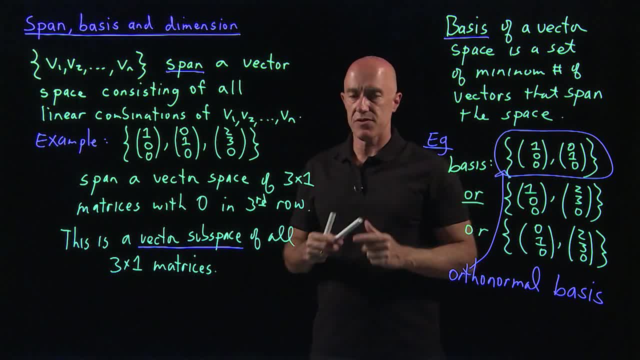 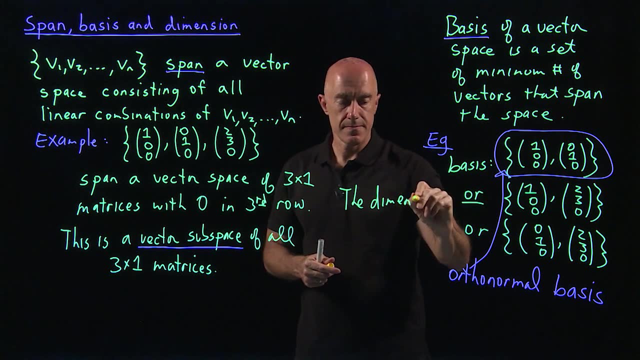 All three of these are valid basis, though, for this vector space. OK, So we've got span, We've got basis. The last one is dimension. So dimension, The dimension of a vector space, is the number of basis vectors. OK, 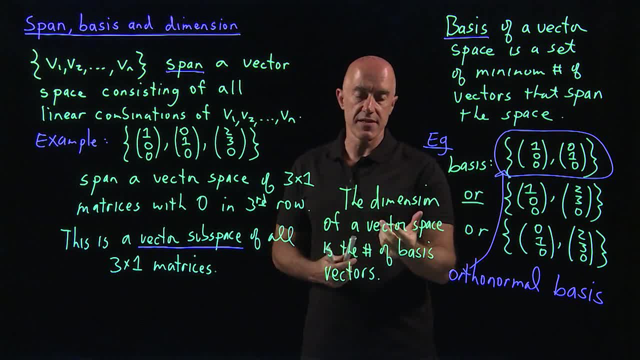 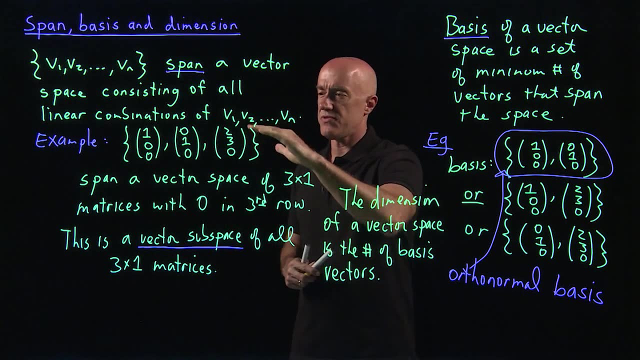 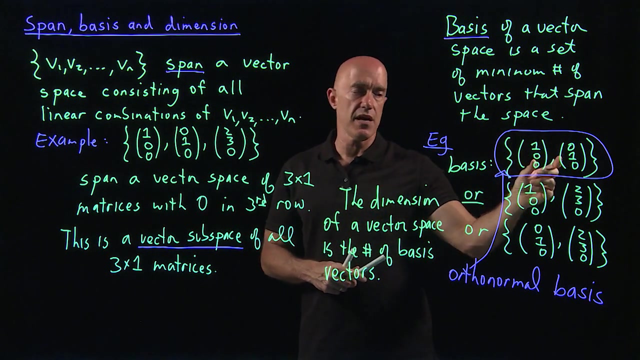 And that's unique. So the number of basis vectors required to span a vector space is given is called the dimension of the vector space. So here the vector space of 3 by 1 matrices, with 0 in the last row, requires two vectors to form a basis for that vector space. 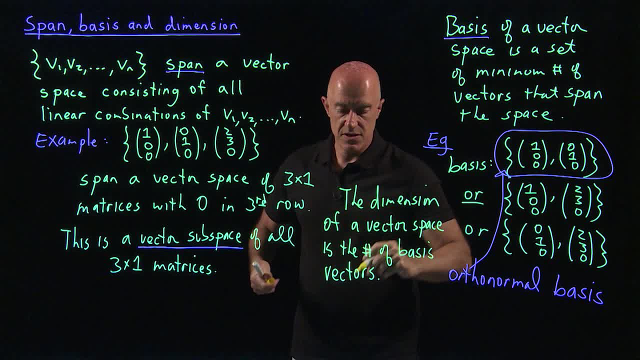 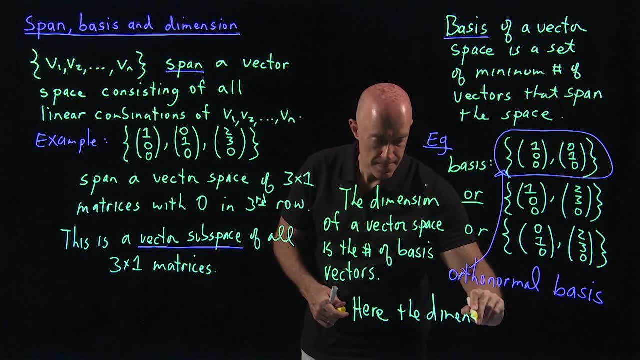 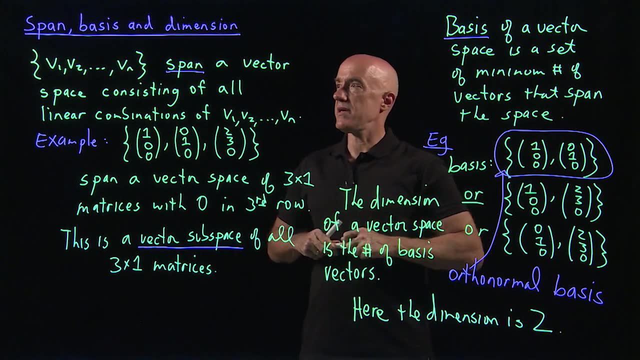 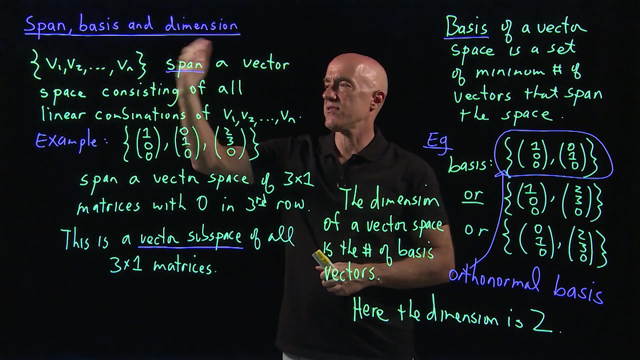 So the dimension of that vector space is 2.. So here the dimension Is 2.. OK, So let me summarize then these definitions. We say a set of vectors span, a vector space consisting of all linear combinations of that set. 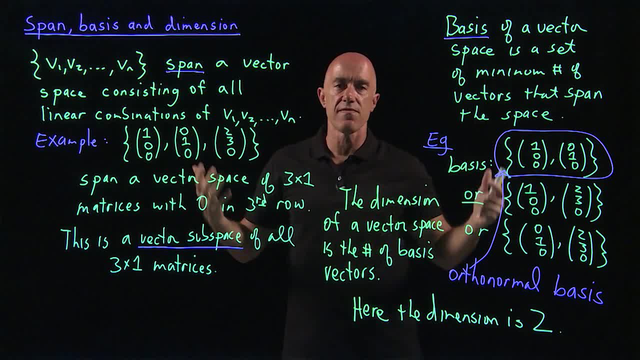 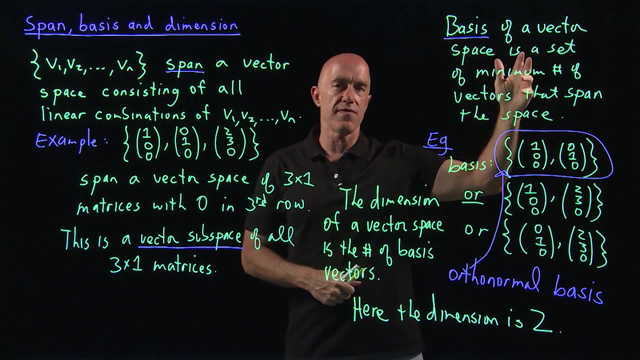 So you can, given any set of vectors, you can form a vector space by forming all possible linear combinations of that set of vectors. But you can condense that more by forming a basis for a vector space. So a basis for a vector space is a set.